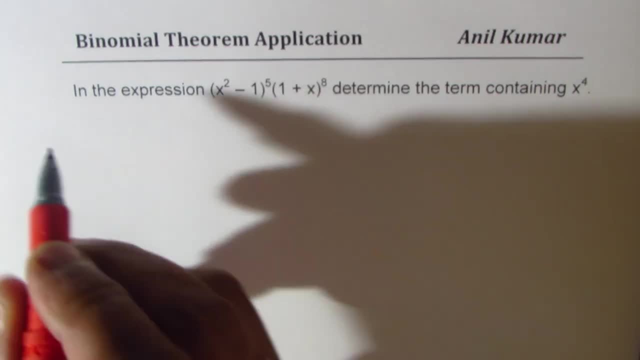 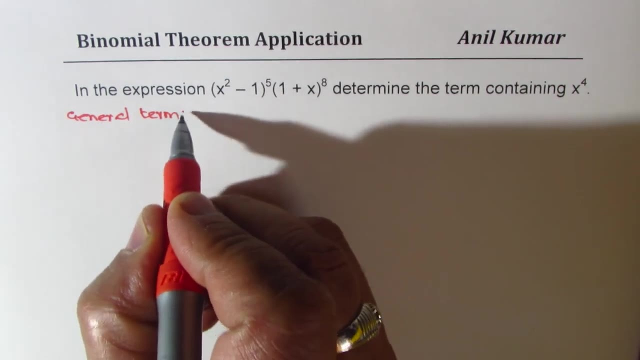 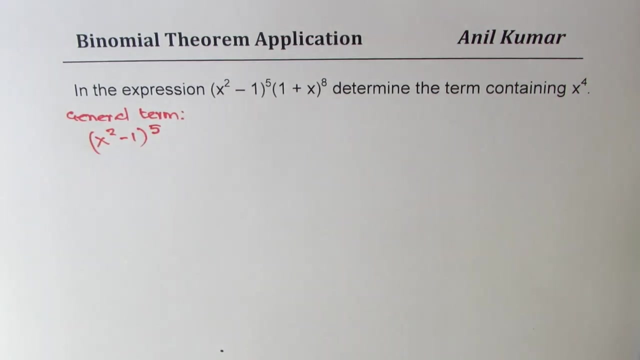 is to find general term for each one of them. So let's find general term for the expression which is x square minus 1 to the power of 8 times 1, plus x to the power of 8 times 1 to the power of 5.. So let this be the first step. So general term for this particular. 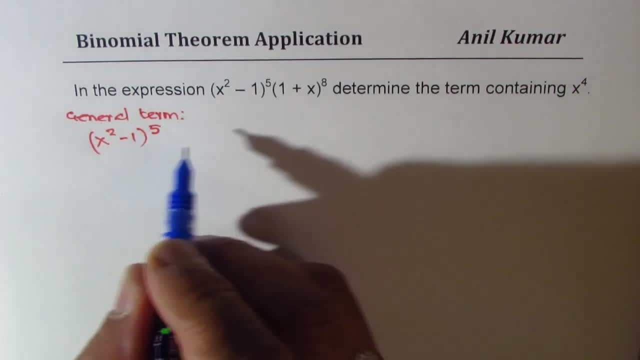 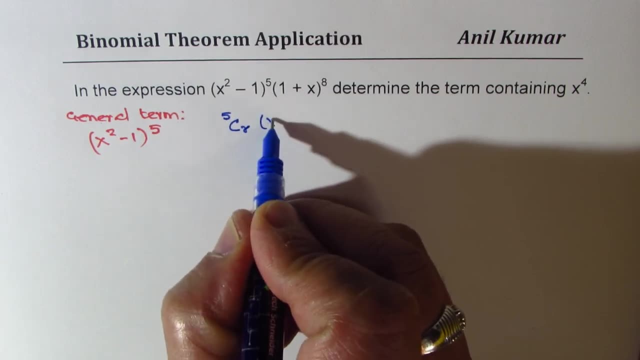 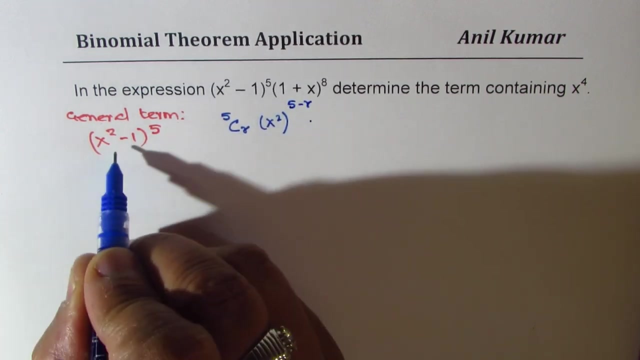 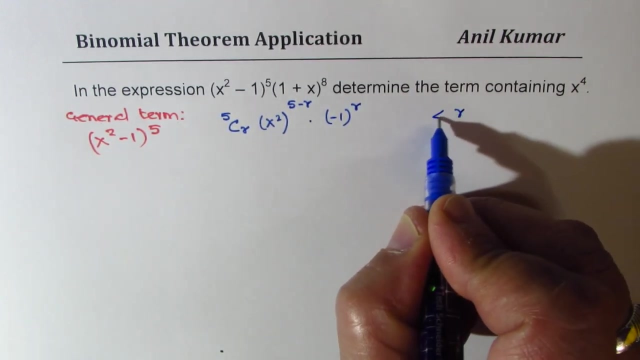 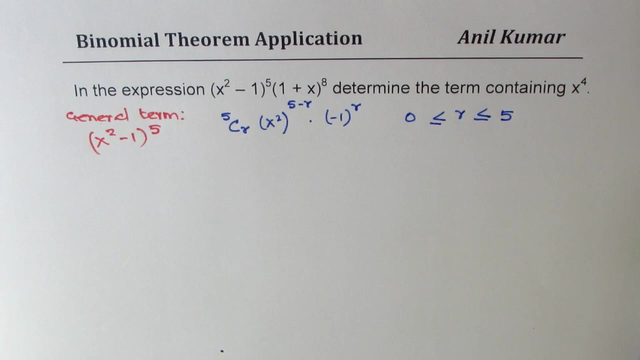 expression will be 5cr x square to the power of 5 minus r, times minus 1 to the power of r. Now, in this case has to be in between the values 0 to 5.. Now, let us now find general term for the second. 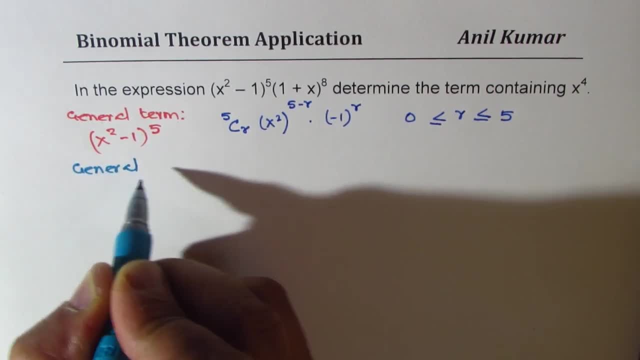 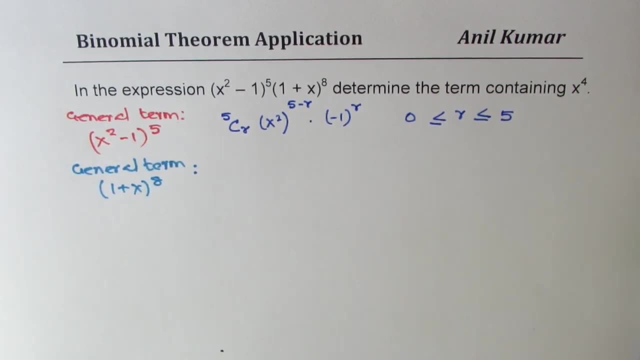 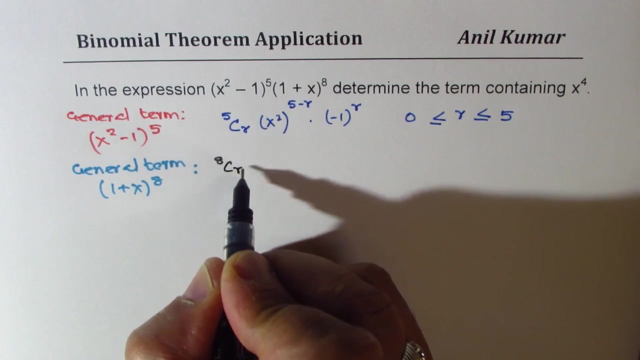 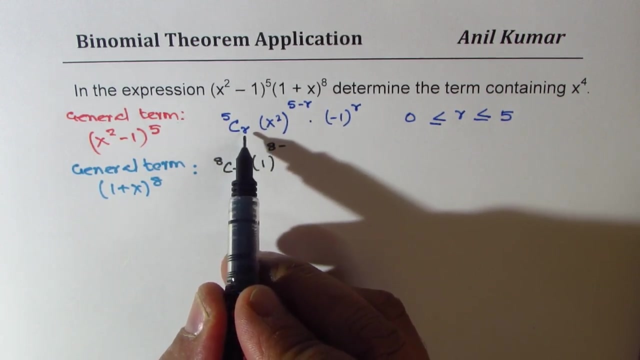 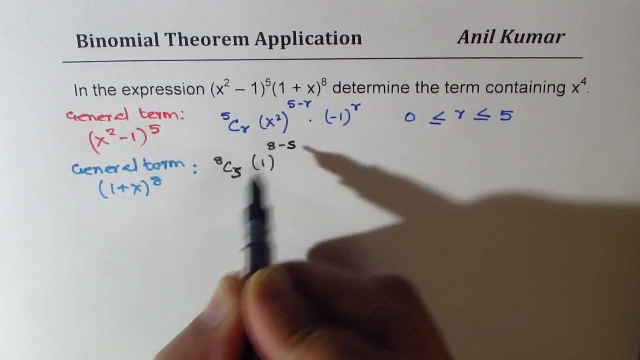 one which is the binomial 1 plus x to the power of 8.. So general term for this will be 8cr, 1 to the power of 8 minus. Now it is better to take some other coefficient right. So instead of r I am going to take s. So I will make 8 minus s. This could be: 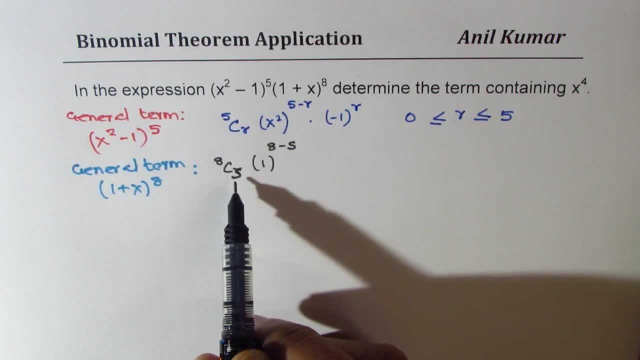 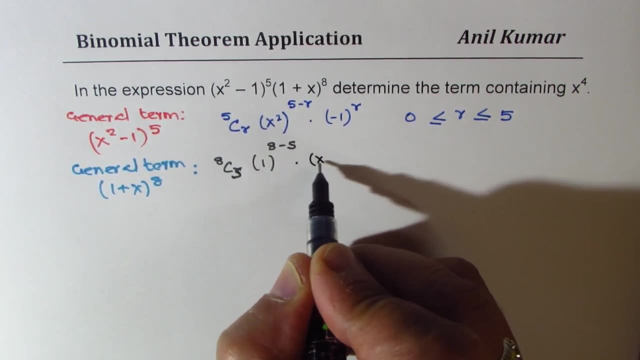 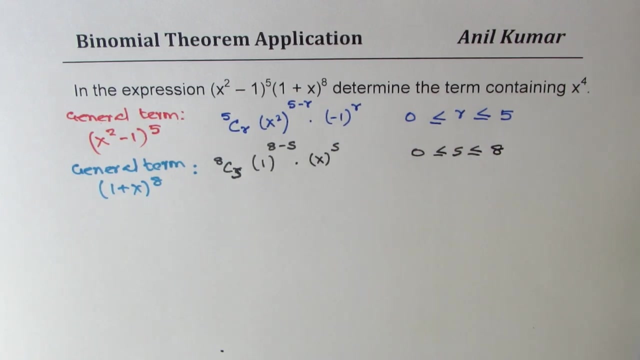 any variable correct. To avoid confusion, we should take some other variable. So 8 minus x, s, x to the power of 8.. Now, where s will be between 0 and 8, right Now, how about the general term for the product? 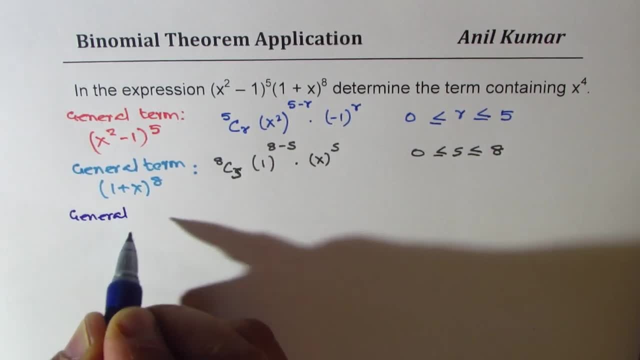 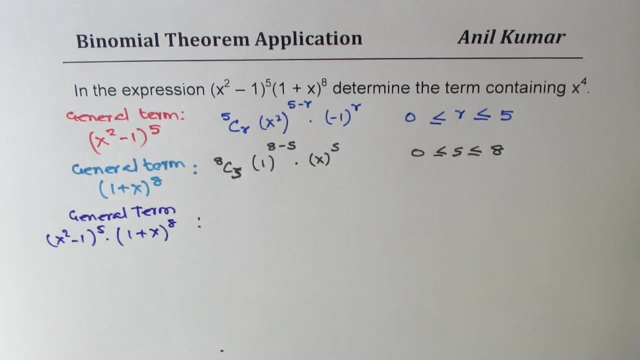 So let us write down the general term for the product, which is, in our case, x square minus 1 to the power of 5 times 1 plus x to the power of 8.. So that is going to be let. 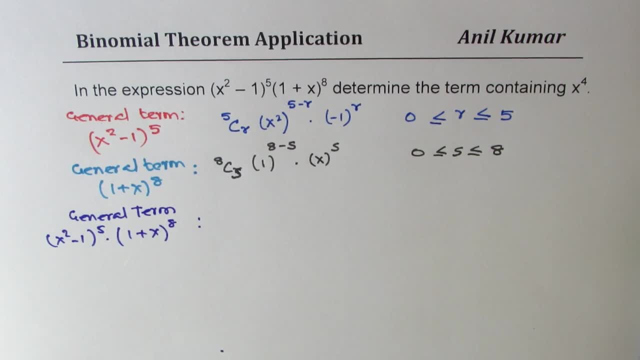 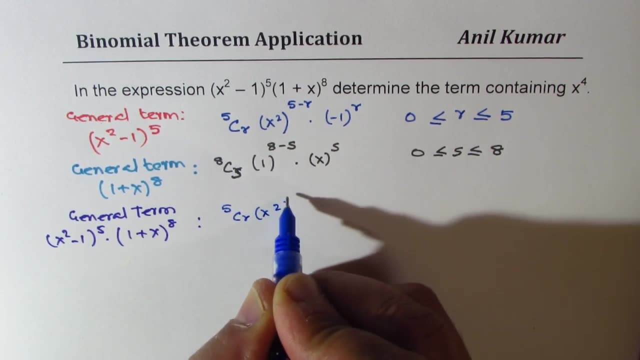 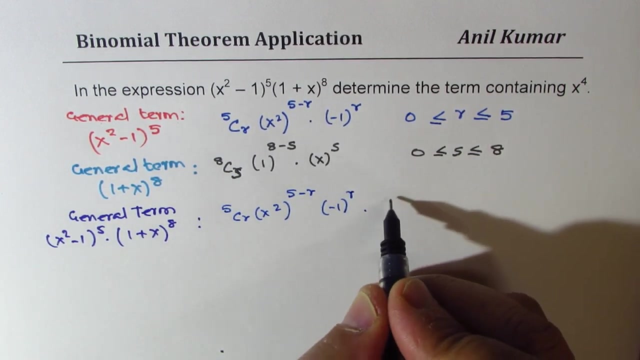 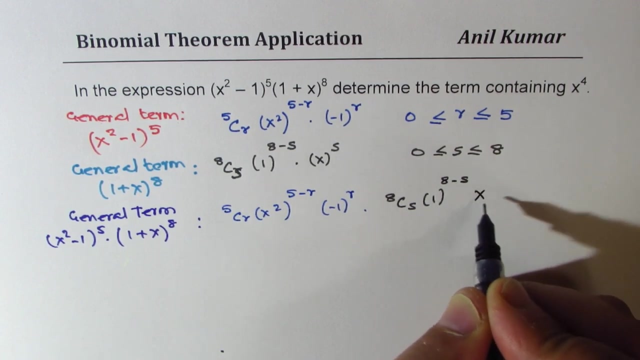 us write down the product of the above terms, right? So let me rewrite that as: 5cr x square 5 minus r times minus 1 to the power of r times. the other term, which is 8cs, 1 to the power of 8 minus s, x to the power of s, Now 1 to the power of 8 minus s, is going to be: 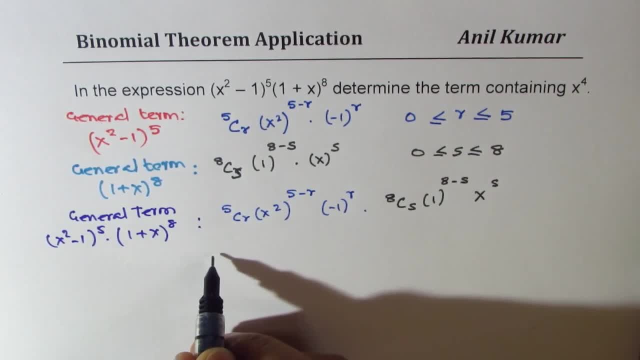 1. So we are kind of neglected. So what we really get here is 5cr times 8cs, x to the power of 2 times. we can multiply this right, So we get 10 minus 2r minus 1 to the power. 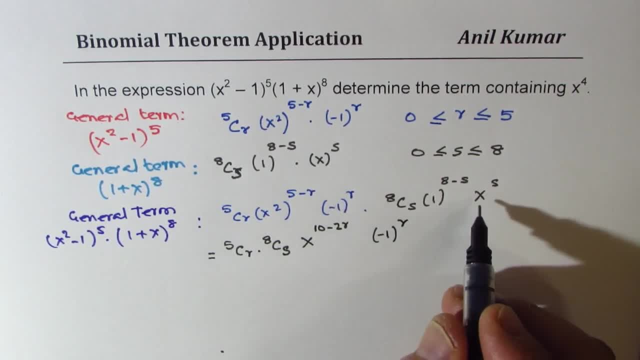 of r, and here we have x to the power of s. Now combine these two terms, right, So we get 5cr times 8cs minus 1 to the power of r, x to the power of these two, right So. 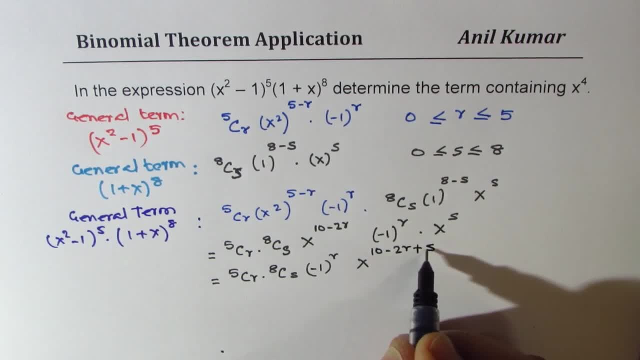 it is 10 minus 2r plus s. Now what we really need is a term containing x to the power of 4.. This is what we need. So what we can equate here is for terms with x to the power of 4, the condition is that the numerator, I mean the exponent which 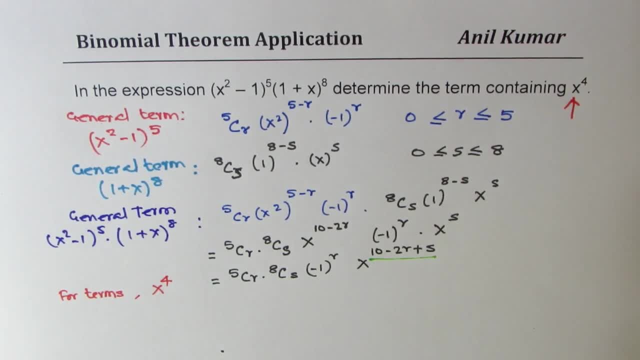 we see here should be equal to 4, right. So that gives you that 10 minus 2r plus s should be equal to 4, right. Solving this: bringing 4 here we get 10 minus 4 equals. 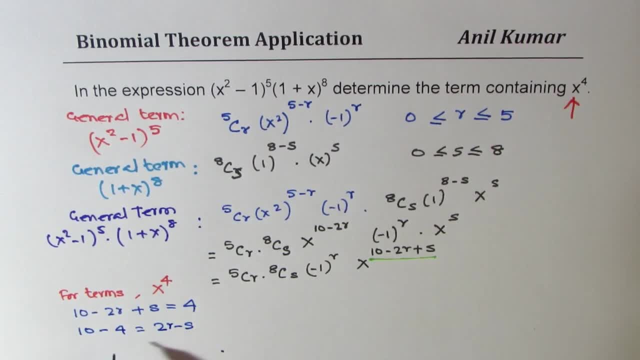 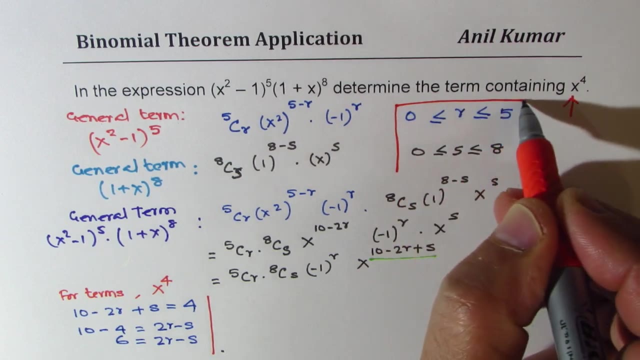 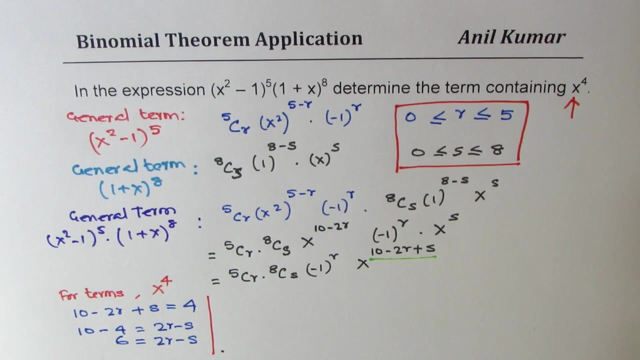 to 2r minus s. or we can write: 6 is equals to 2r minus s. So we have now an equation which relates r and s. Remember the value of r and s could be as shown here Now to get 6, let me rewrite the equation here and find possible values. So what we are looking 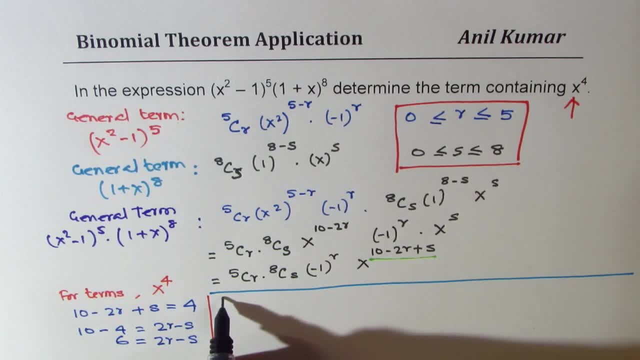 for now is solution for the equation: 2r minus s equals to 6.. We know that r is within the interval 0 to 5 and s is within the interval 0 to 8. So we are looking for all possible solutions. 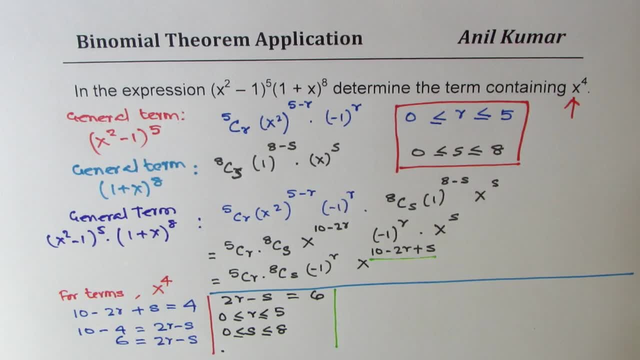 A combination of r and s. That's the whole idea. right Now, since we have to take away the value of s, r could be 3.. So if r equals to 3, then we get 6 minus 0 we could use. 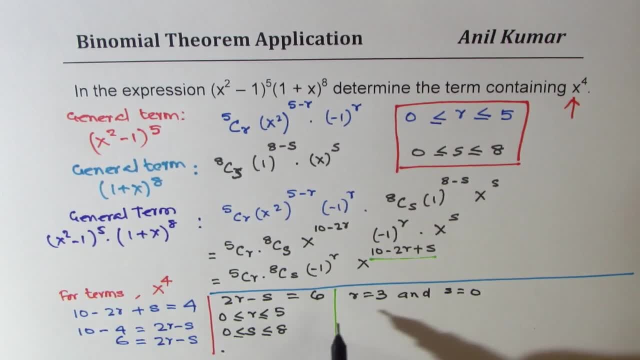 So and s equals to 0 gives us one solution. Well, r could be 4.. If r is 4,, it is 8.. 8 minus 2 is a solution. So and s equals to 2 will be a solution. 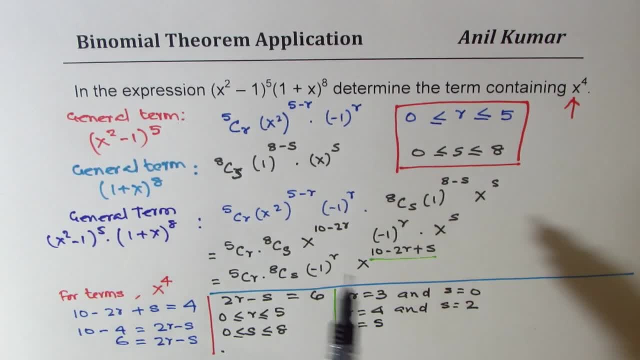 How about R equals to 5.. If I put that's the maximum value which r can have 5 times 2 is 10, 10 minus 4.. So and s equals to 4 will also give us a solution, right. So these are the possible. 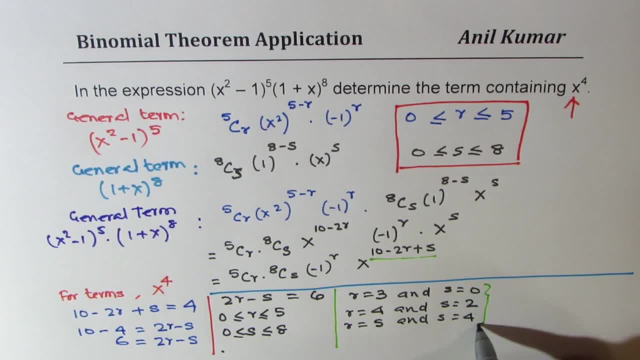 solutions. right, So that gives you all possible combinations For x to the power of 4, right? So what we need to do is to collect all these terms combined and get our answer correct. So let's move on and calculate. So the general term which? 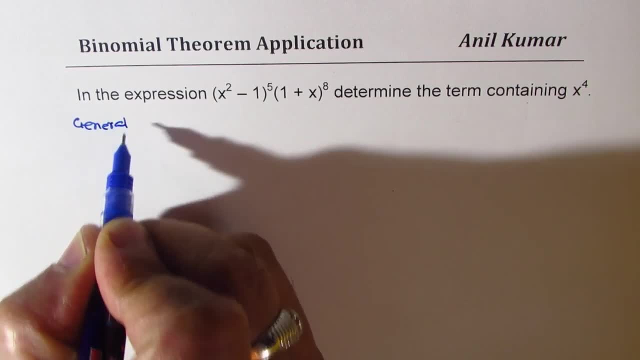 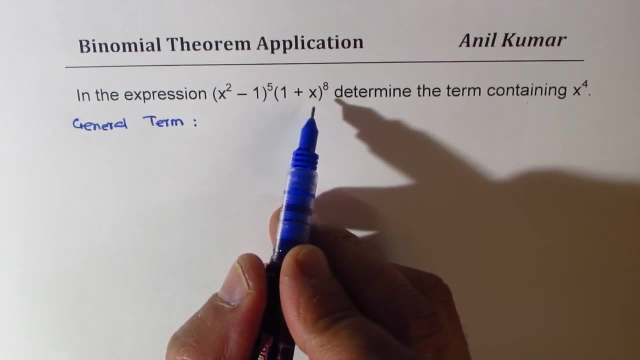 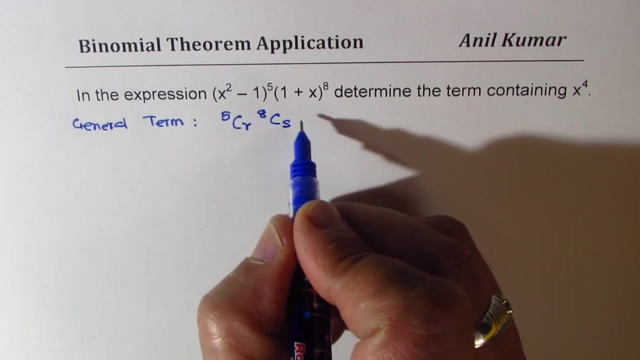 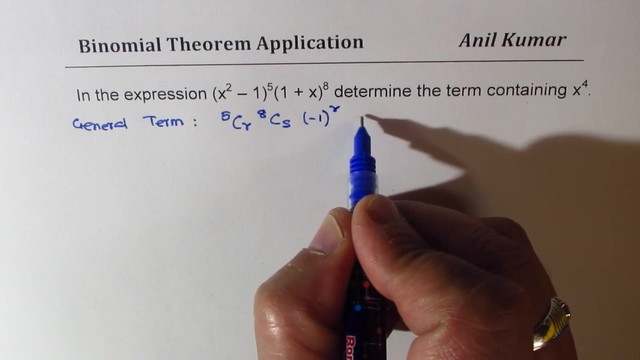 we got was kind of like this: Let me rewrite For this expression: with x to the power of 4, which we just calculated is 5cr 8cs minus 1 minus 1 to the power of r times x to the power of. So we are talking for. 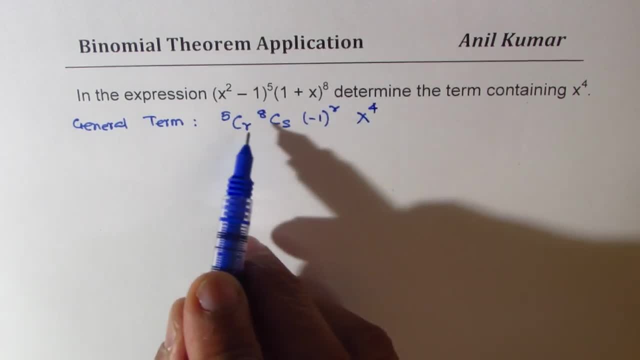 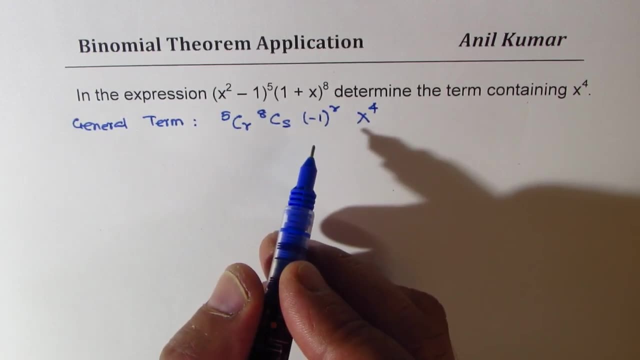 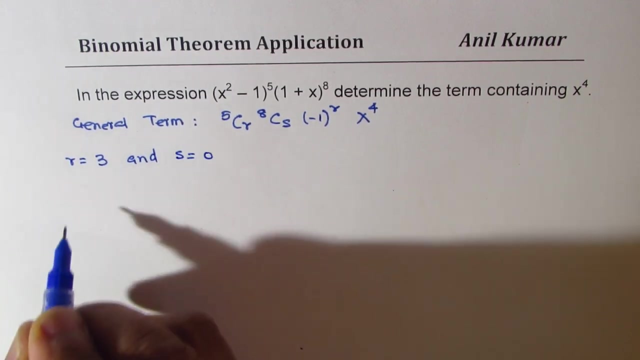 a general term, with x to the power of 4, right. So for this particular condition, where x is to the power of 4, we got combinations of r and s, as r equals to 3 and s equals to 0.. We also got r equals to 4 and s equals to 2, and we got r equals to 5 and s equals to. 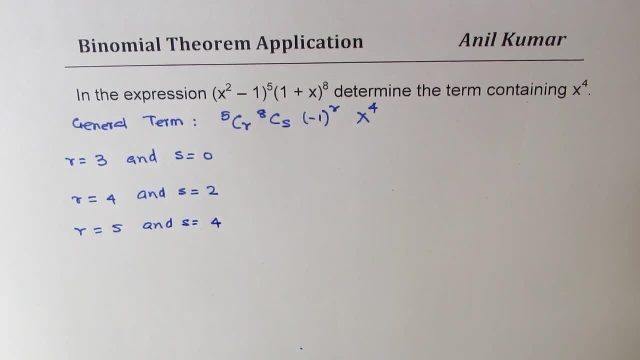 4, right. So these were the 3 possible solutions which we got. Now, for each one of these, let us calculate the terms, right. So for each one of these, let's calculate the terms. So for the first one, 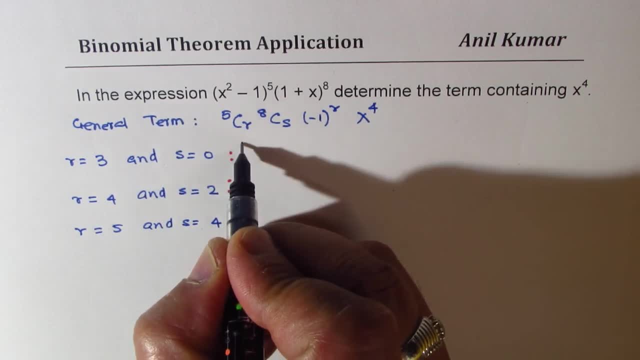 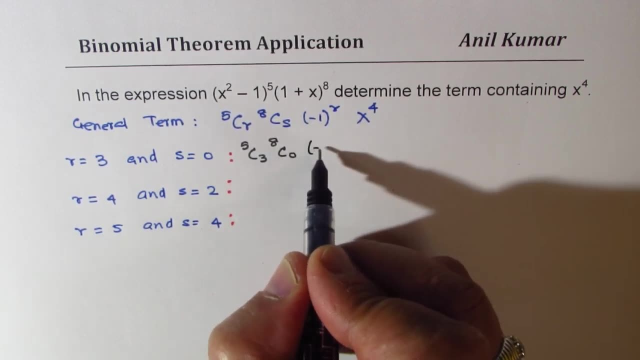 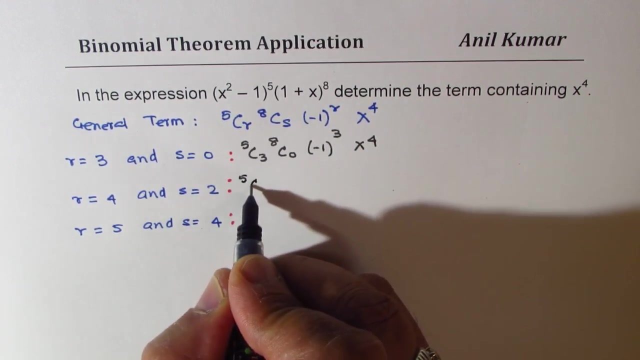 okay, we get r equals to 3, where r is 3, we get 5c3, 8c0, minus 1 to the power of 3, as x to the power of Correct. For the second one, we get 5c4, 8c2, minus 1 to the power. 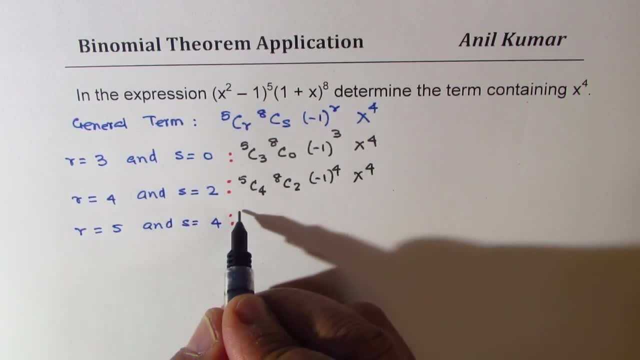 of 4 times x to the power of 4. and for the last one, we get 5c5, 8c5, minus 1 to the power of 3 times x to the power of 4.. Okay, Don't forget to. 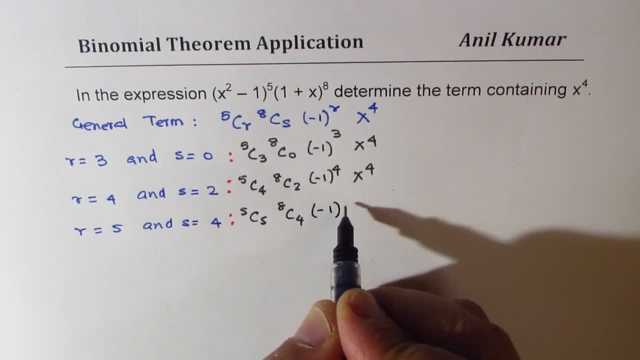 8 c, 4 minus 1 to the power of 5, x to the power of 4. okay, so these are the three terms which will have x to the power of 4 in it. so the first term here is negative power. 4 will make this positive and the third term will be negative. right now let's calculate. 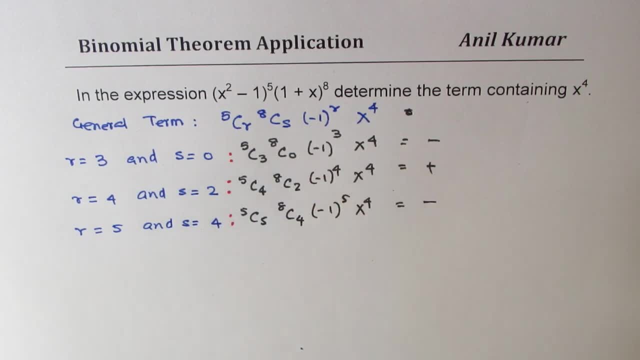 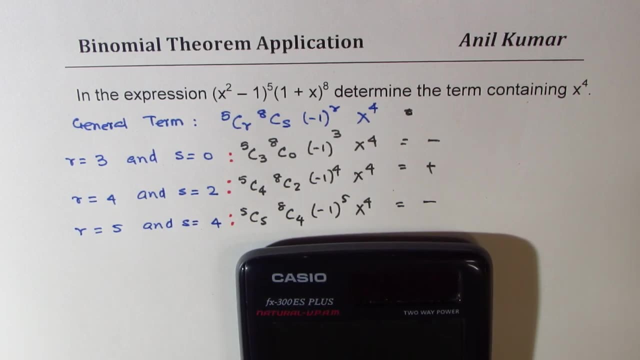 these values 5 c 3, 8 c, 0. so we can use the calculator to calculate. well, some of you can directly find the answer using the formula you know. so we'll calculate: 5 c 3, 5 c 3 times 8 c. 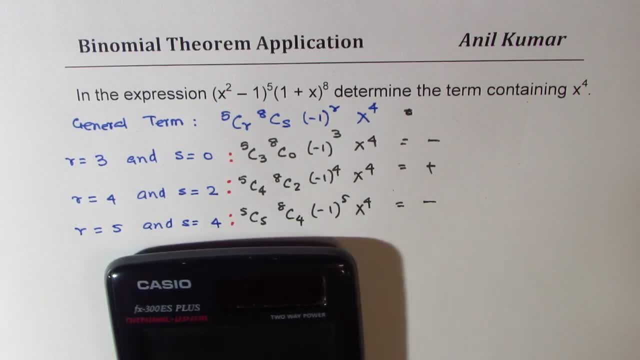 0 equals to 10, so we get this as 10 x to the power of 4. then we have 5 c 4, 5 c 3. x to the power of 4, 5 C 4 times 8 C 2, 8 C 2, which is 140 X to the power of 4. and the last term here: 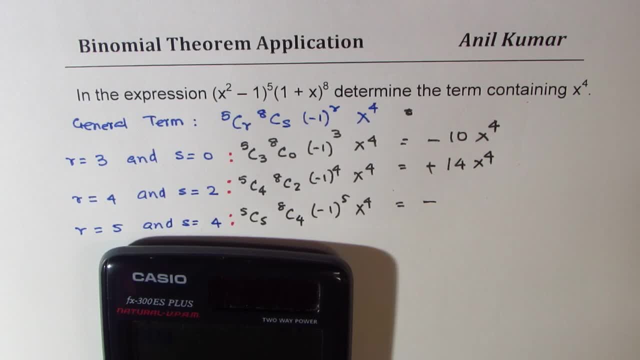 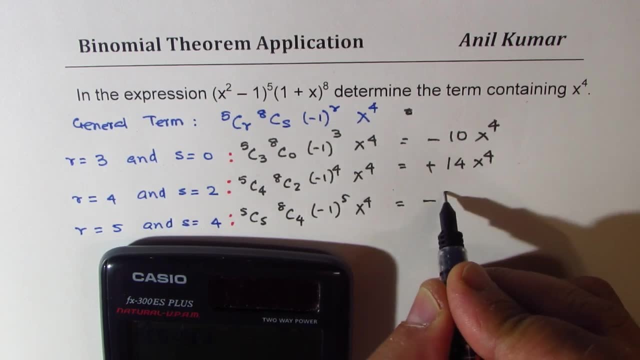 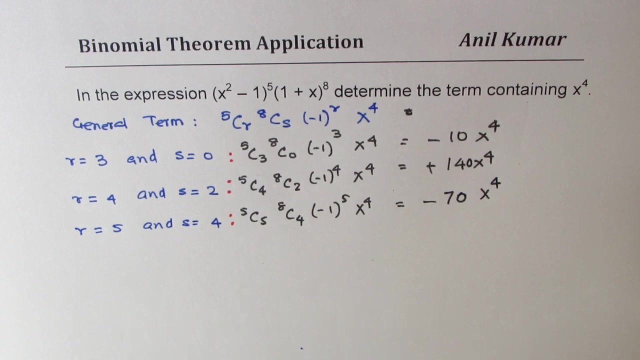 is 5 C 5 times 8 C, 4, which is equal to 70 forward to write 0 here: X to the power of 4. so these are the three terms which we get. now, combining these three, we get our answer right. so the term with X to the power of 4. so the coefficient: